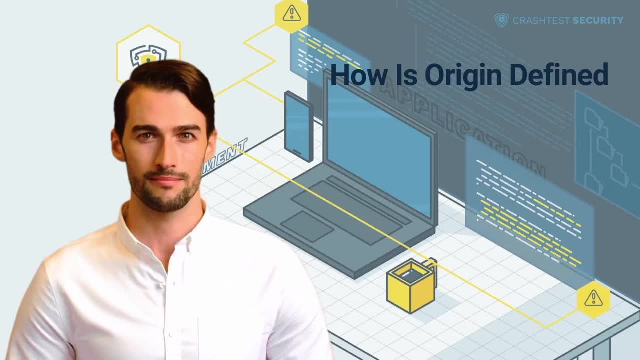 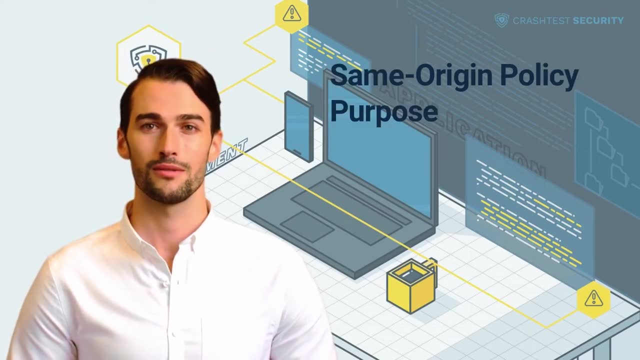 would and would not be considered the same in our blog post. Whether the origin is the same or not affects how browsers treat requests between origins. The purpose of the SOP is to regulate whether and how origins and their resources interact. It is implemented on the web and it is used for the purpose of regulating whether and 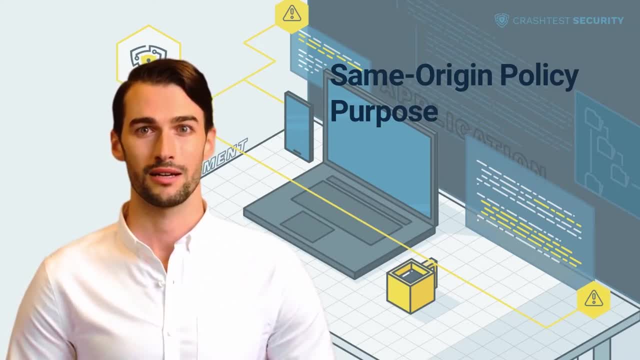 the browser level to guarantee no unauthorized cross-origin communication that could lead to a malicious script on one website obtaining access to sensitive data on another. Or, to put it differently, it prevents the reusing of authenticated user sessions across websites and read access to responses from different origins When a client sends a request to an. 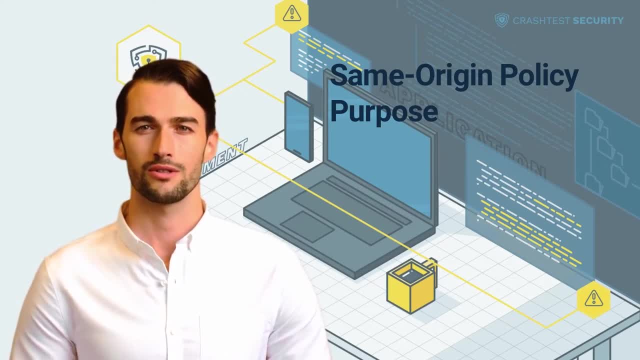 origin. the request includes authentication details, such as session cookies, relevant to that origin. Imagine: a user is tricked into visiting a website with a misleading domain that contains a frame that loads the contents of the actual website. The user then proceeds to log in and, in doing so, sends the necessary authentication cookies to the actual domain via. 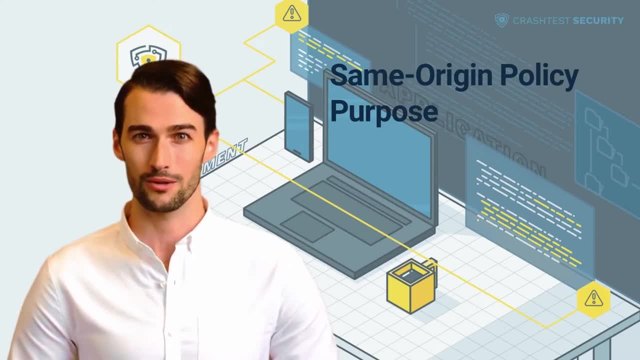 the malicious website. If there were no same-origin policy, the response of the actual website could be read by attackers. It would enable them to access the user's data via the document-object model of the actual website and make requests on their behalf. Thanks to the same-origin policy, this is not possible. 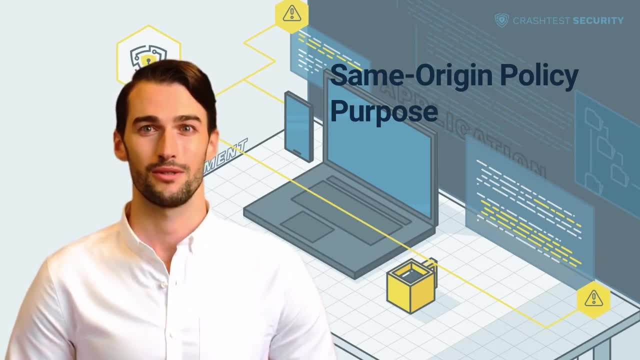 What does the same-origin policy do? origin policy forbid and allow. The SOP is sometimes erroneously understood as blocking all kinds of cross-origin requests. If that were the case, it would not be possible to serve resources between origins and there would be no point in the existence of content delivery networks. 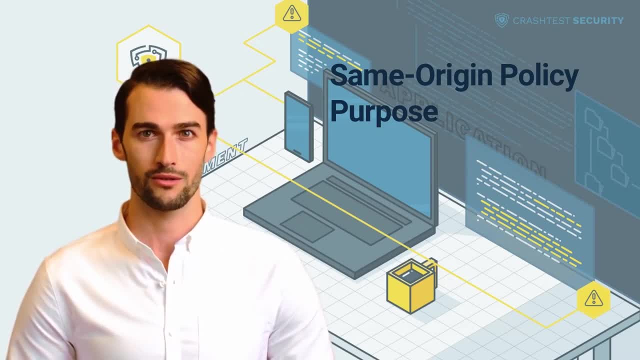 and even the web. Neither does the SOP forbid origins from making requests to each other or writing between origins, such as submitting forms. Broadly speaking, the SOP allows resources to be embedded, but does not allow cross-origin reading. The difference between embedding and 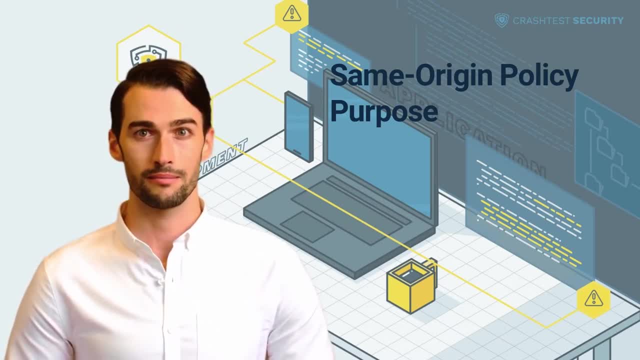 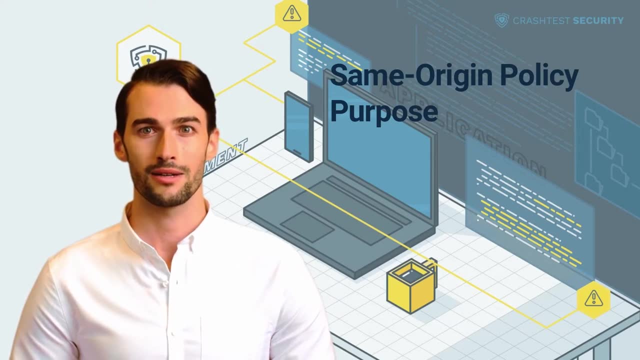 reading is that an embedded resource is copied and becomes independent of its origin, whereas with reading, the external origin is preserved. Permitted forms of embedding include hang tags such as iframe, script, em, video, audio link, object: embed and form. This part of the POS can 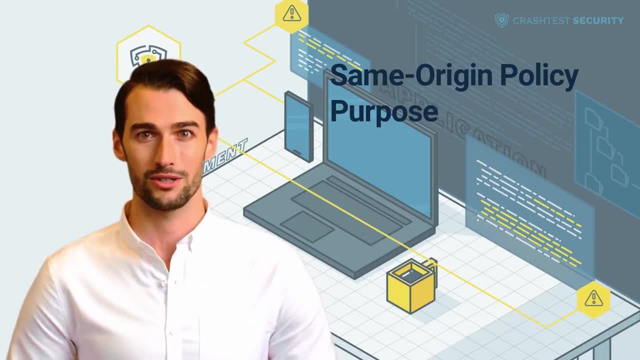 sometimes be a source of security vulnerabilities and lead to clickjacking attacks. There are differences in the SOP. The SOP application varies between technologies and resources, such as cookies, JavaScript, DOM and other APIs. That said, here are a few examples of what SOP will typically. 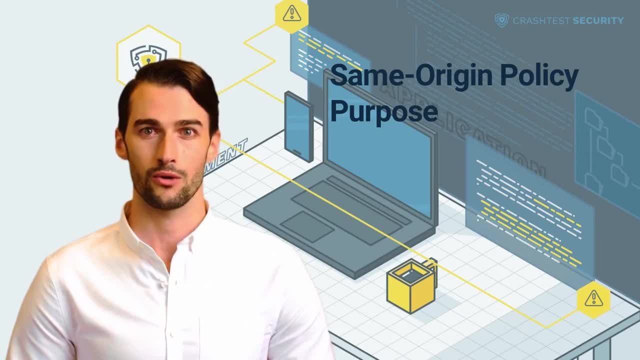 forbid. Cookies cannot be sent to a page with a different origin, though in this case this only applies to pages with other domain subdomains. whereas schema and port are not checked, AJAX requests, such as XML HTTP request, are not allowed under SOP. 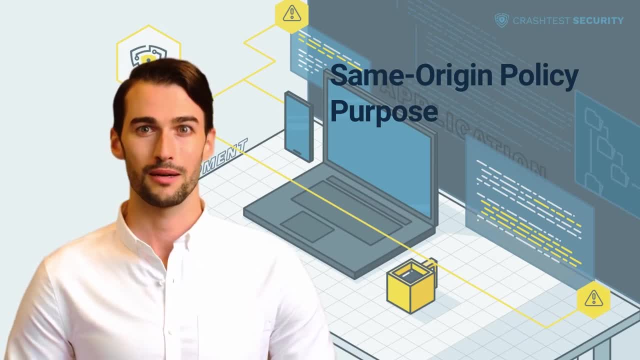 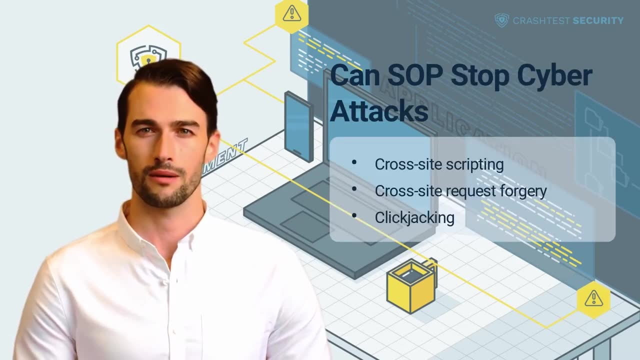 though this is possible if cross-origin resource sharing is implemented. Even when embedded, JavaScript cannot read content on a website with a different origin. While SOP is highly useful in preventing several types of attacks, it has its limits and cannot contain all cross-origin threats. The main threats associated with exploiting origin vulnerabilities: 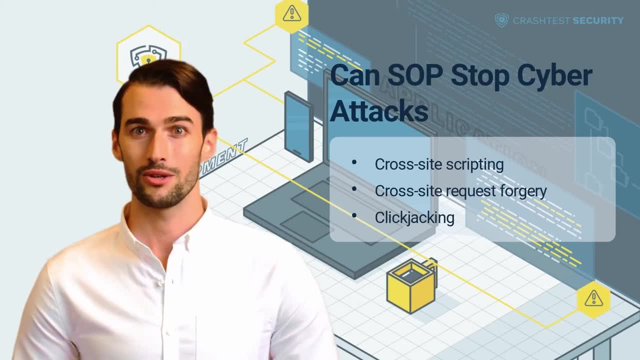 are cross-site scripting, cross-site request forgery and clickjacking attacks mentioned above. Cross-site scripting includes injecting malicious code on the client side to force the browser to perform specific actions and steal sessions. Cross-site request forgery relies on a user visiting a malicious website with an embedded 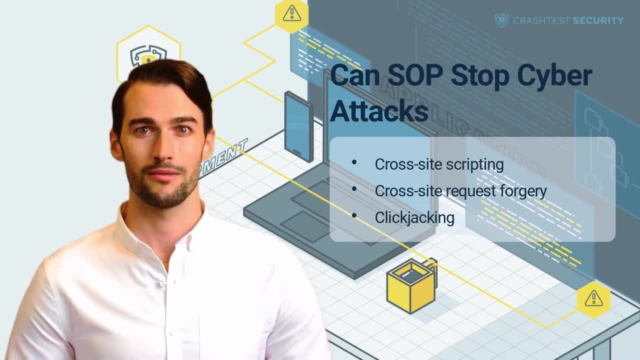 code that begins to generate requests on behalf of the user without their knowledge. Clickjacking is the use of transparent buttons on top of an embedded frame. These buttons link to malicious websites where users' sessions and data can be stolen or hijacked. It would be best if you took additional actions that the SOP does not cover to prevent these. 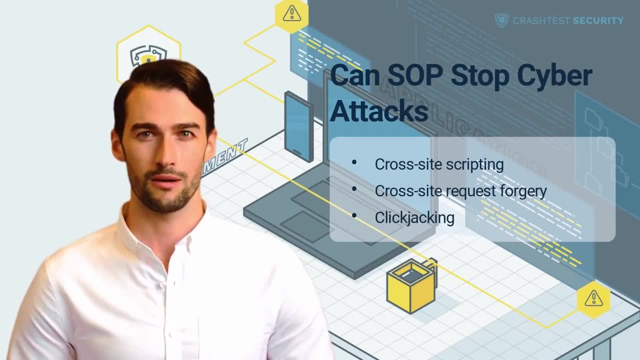 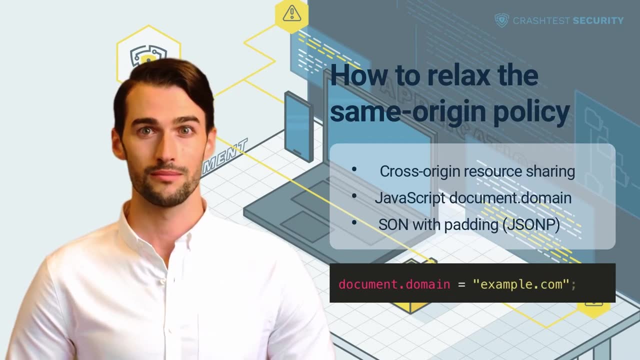 attacks: See the pages associated with these attacks. The policy-strict rules can create difficulties for websites that have multiple subdomains or when two domains should be able to interact. There are ways in which cross-origin communication can be enabled in a controlled manner in such situations. 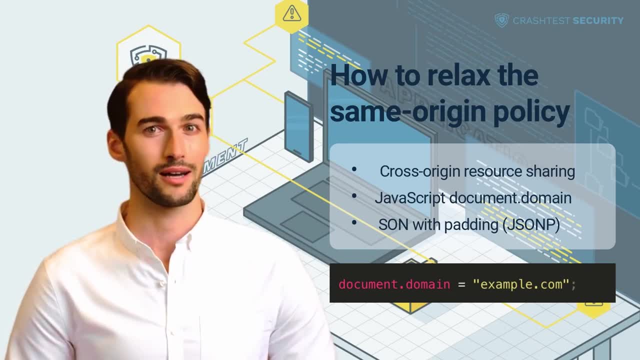 Cross-origin resource sharing. One common way of relaxing SOP is through cross-origin resource sharing. CRS enables the sharing of external resources through the HTTP access control. allow origin response header. A browser sends a request header to a different origin and the server provides the necessary instructions in its response header If, according to the instructions, the request from 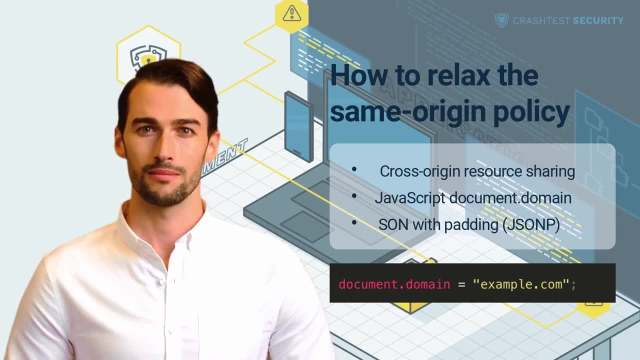 this origin is permissible, the browser allows the server response. If not, the answer is not shared by the browser. CRS also offers the possibility to perform a preflight request, also known as an options request. The preflight request asks the server whether it will permit the client.